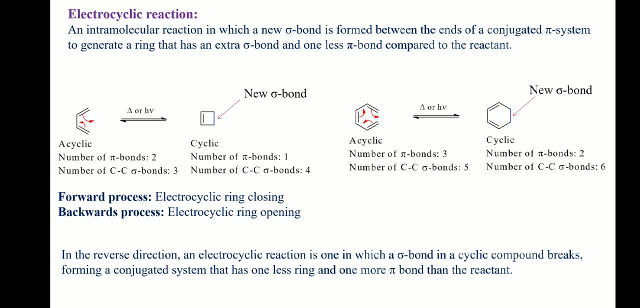 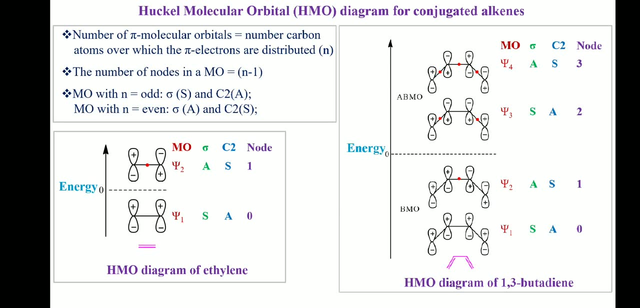 cyclohexadiene reaction. To learn more details of electrocyclic reactions, we need to learn how to construct Huckel molecular orbital diagrams of different pi electron systems and different terminologies used in the electrocyclic reactions. Huckel molecular orbitals of ethylene and any. 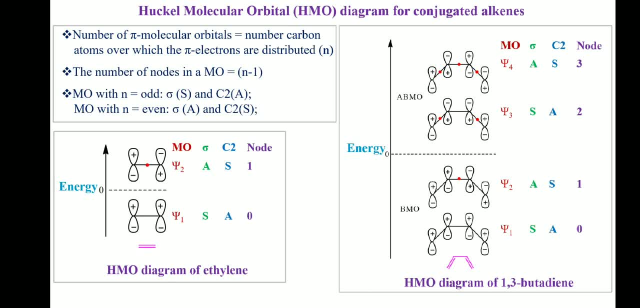 conjugated alkene can be constructed if we remember these three points. Number of pi molecular orbitals is equal to the number of carbon atoms over which the pi electrons are distributed. The number of nodes in a molecular orbital is equal to n-1, where red dots represent: 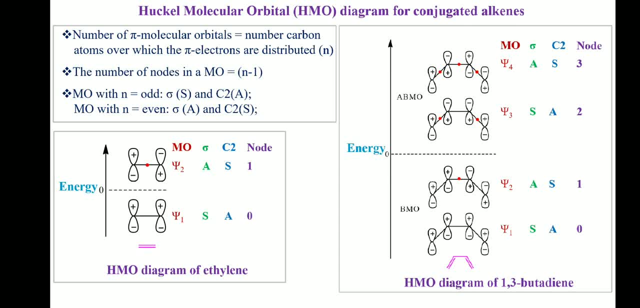 nodes. Molecular orbital with n is equal to odd, has plane of symmetry and does not have C2 axis of symmetry, while molecular orbital with n is equal to even, has C2 axis of symmetry and does not have any plane of symmetry. We are first going to discuss Huckel molecular orbital diagram of. 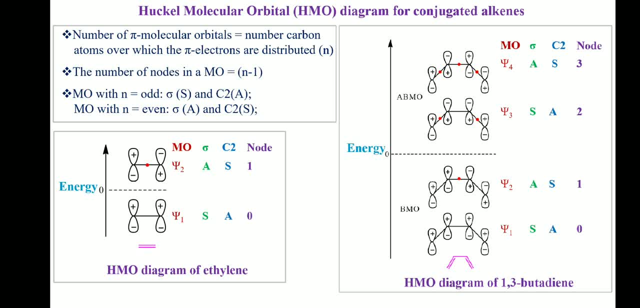 ethylene, which is the simplest alkene. In ethylene there are two carbon atoms over which the pi electrons are distributed. So the pi electrons are distributed over the pi electrons. The number of pi molecular orbitals will be two Out of two, one represented by psi-1 below the 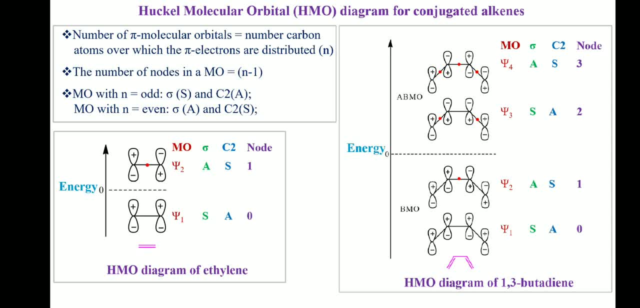 dashed line is bonding, while other, represented by psi-2 above the dashed line, is antibonding. Psi-1 with n is equal to odd, has plane of symmetry and does not have C2 axis of symmetry, while psi-2 with n is equal to even, has C2 axis of symmetry and does not have C2 axis of symmetry. 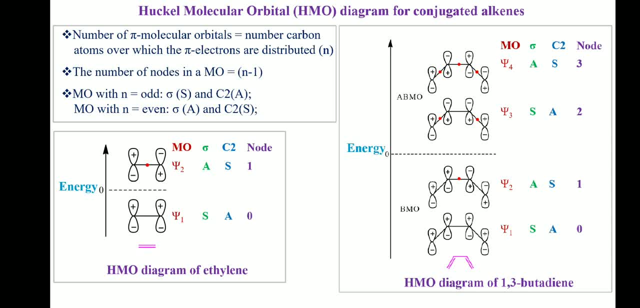 According to the n-1 rule, psi-1 with n is equal to 1 has zero node, while psi-2 with n is equal to 2 has one node, where the red dots represent node In the case of 1,3-butadiene. 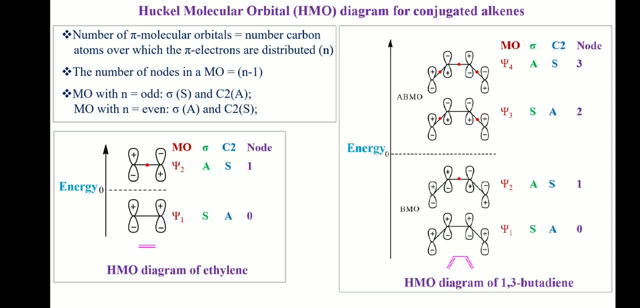 there are four carbon atoms over which the pi electrons are distributed, So the number of pi molecular orbitals will be four. Out of four, two, represented by psi-1 and psi-2, below the dashed line are bonding, while the remaining two, represented by psi-3 and psi-4 above the dashed line, are antibonding. 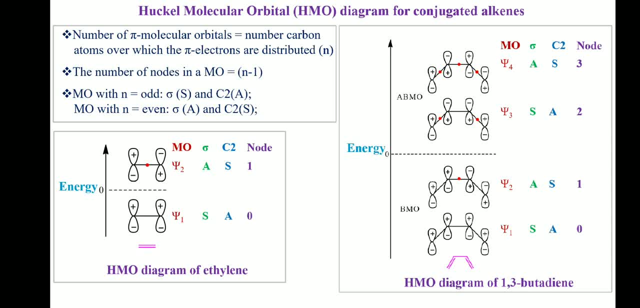 Psi-1 and psi-3 with n is equal to odd, have plane of symmetry and do not have C2 axis of symmetry, while psi-2 and psi-4 with n is equal to even have C2 axis of symmetry and do not have plane of symmetry. 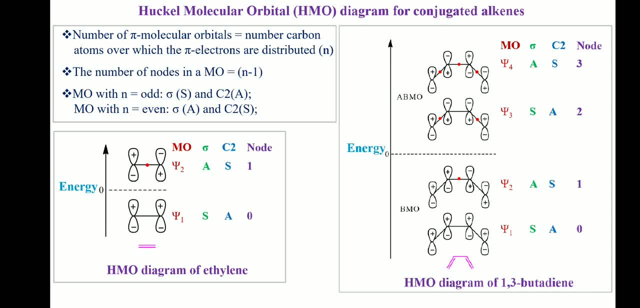 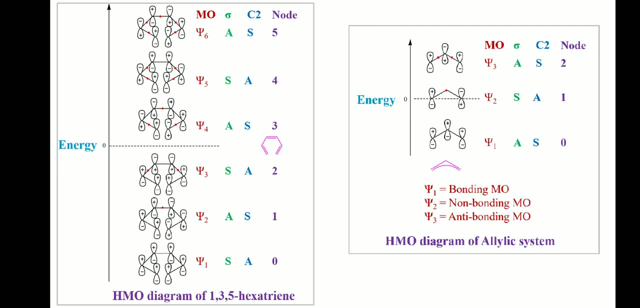 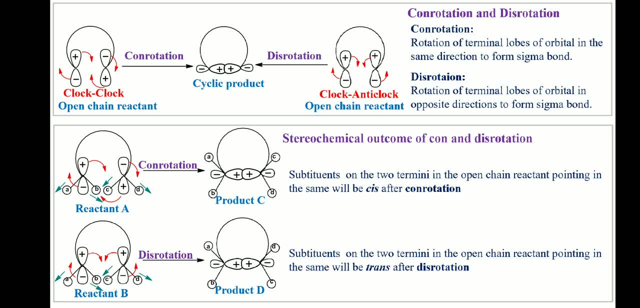 Conrotation and Disrotation are the two terms frequently used in electro-cyclic reactions. These two rotations govern the stereochemical outcome of an electro-cyclic reaction, So the proper understand out of these two terms is essential for the better understanding of electro-cyclic reactions. 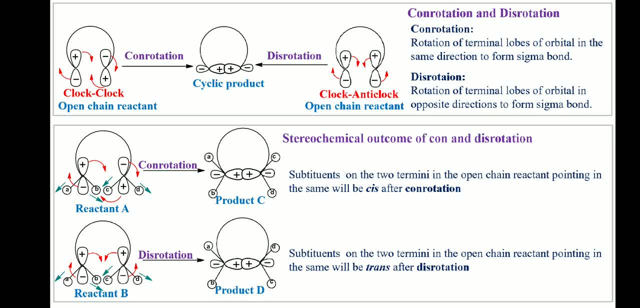 In con rotation the terminal lobes of highest occupied molecular orbital of open chain reactant rotate in the same direction, either clockwise or anticlockwise, to form product, while in this rotation the terminal lobes of highest occupied molecular orbital of open chain reactant 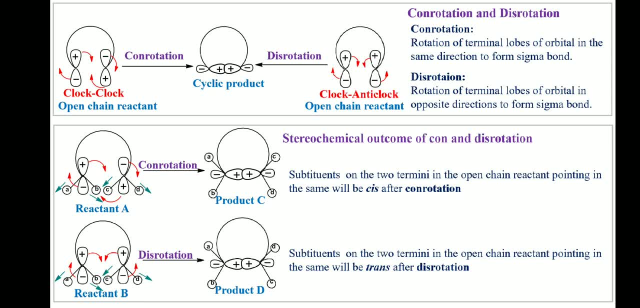 rotate in opposite directions, one clockwise and other anticlockwise, to form the product. Let us discuss how these two rotations affect the stereochemical outcome of an electrocyclic reaction. Suppose we have two reactants, A and B, such that, under given condition, A undergoes con. 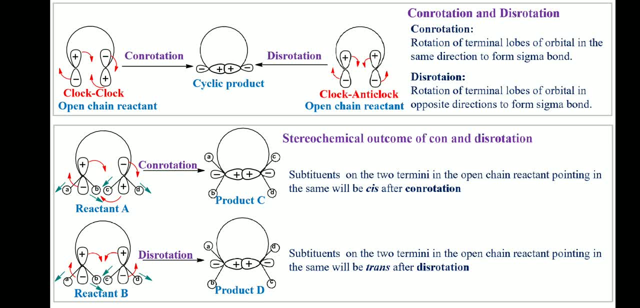 rotation while B disrotation. The two groups A and B on the left terminus are respectively pointing in the same direction than the groups C and D present on the right terminus. Reactant A after con rotation gives product C. If we see the relative stereochemistry of groups A, B, C and D, we will find that in 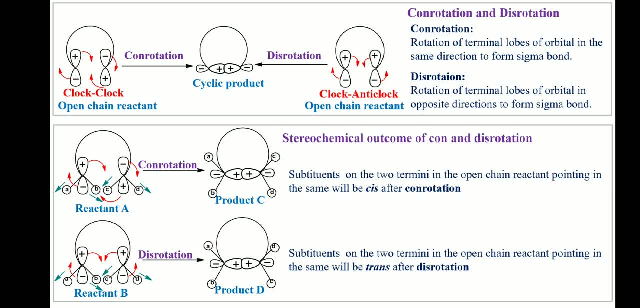 the product. C groups A and B are respectively cis to C and D like reactant. So we can make a generalized statement that after con-rotation, two groups present on the two terminal loops of open chain reactant pointing in the same direction will be cis in the cyclic product. 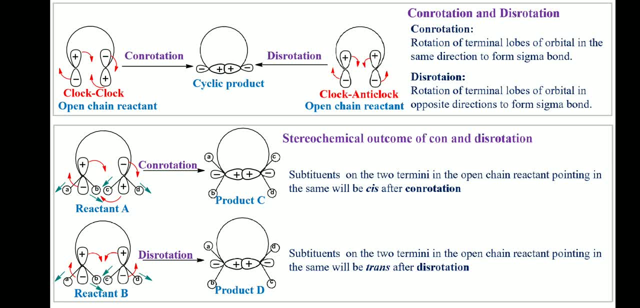 and those pointing in the opposite direction will be trans Reactant. B after dis-rotation gives product D. If we see the relative stereochemistry of groups A, B, C and D, we will find that in the product D groups A and B are respectively trans to C and D. 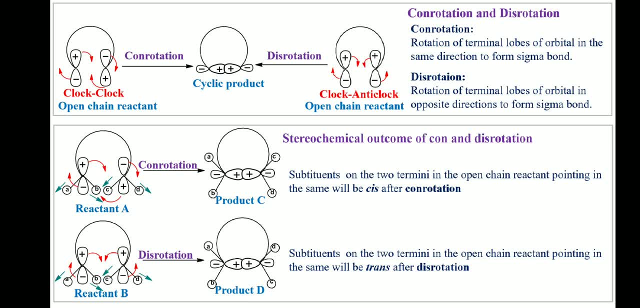 So we can make a generalized statement that after dis-rotation, two groups present on the two terminal loops of open chain reactant pointing in the same direction will be trans in the cyclic product and those pointing in the opposite direction will be cis Woodward-Hartman rule. 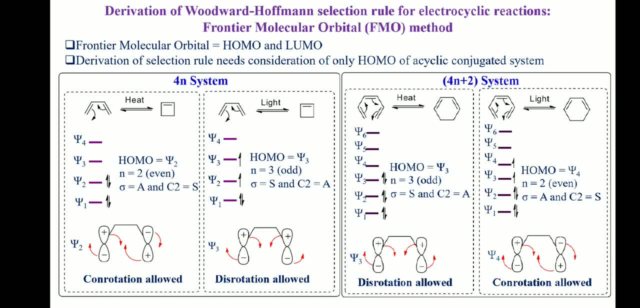 Woodward-Hartman rule is a rule by which we can predict whether there will be a con- or dis-rotation in an electrocyclic reaction under the given condition. There are several methods for the derivation of Woodward-Hartman rule for the electrocyclic reactions. 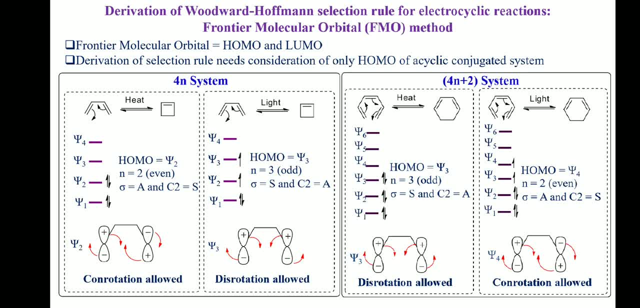 The simplest method is Frontier Molecular Orbital Method. This is also called FMO method. FMO are known as Frontier Molecular Orbitals. Derivation of Woodward-Hartman rule for electrocyclic reaction needs consideration of only HOMO of acyclic conjugated system. 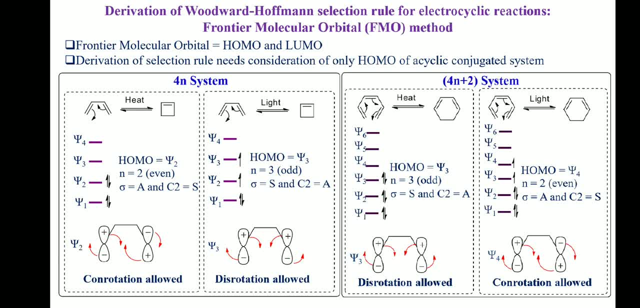 In the beginning we have learned how to construct Hackel Molecular Orbital diagram of ethylene and different conjugated polygons. We don't need to remember everything from that For the derivation of selection rule for electrocyclic reactions, Only the things which we need to remember. 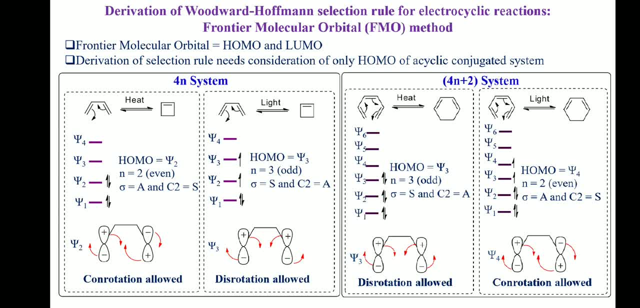 is that the number of Huckel molecular orbital is equal to the number of carbon atoms over which the pi electrons are distributed. Molecular orbital with n is equal to odd, has sigma plane and does not have c2 axis of symmetry, while molecular orbital with n is equal to even. 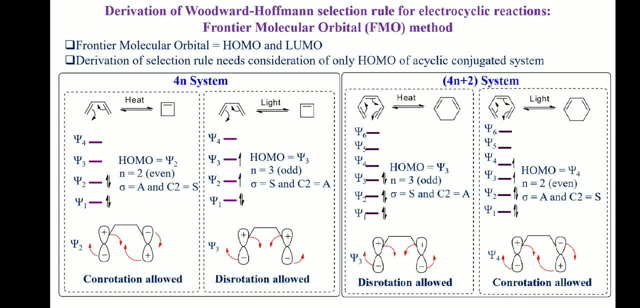 has c2 axis of symmetry and does not have plane of symmetry. We need to take care of the orientation of orbital lobes. only on the terminal carbons Let us derive the Woodward-Huffman rule for 4n pi system. For this we are taking cyclization of 1,3-butadiene to cyclobutene. 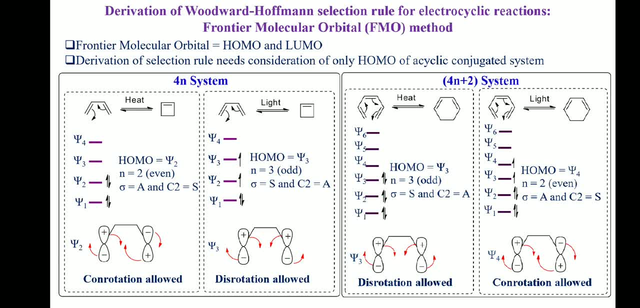 as representative example, In 1,3-butadiene there are four Haeckel molecular orbitals: psi 1, psi 2, psi 3, and psi 4, and 4 pi electrons Under thermal condition. psi 1 and psi 2 are fully occupied, while psi 3 and psi 4 are. 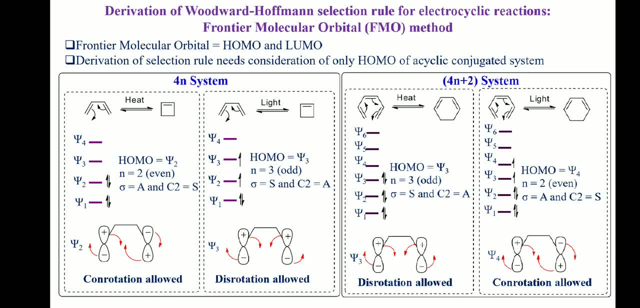 fully vacant. So under thermal condition psi 2 will be homo, Since n is equal to even for psi 2, so it will have C2 axis of symmetry and will not have sigma plane, Since we need to take care of the orientation of orbital lobes only on the terminal carbons. 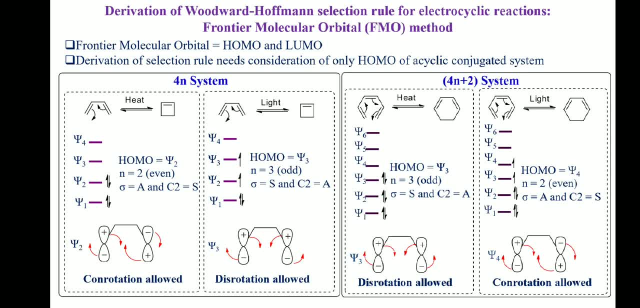 so psi 2 can be represented like the way shown here. The structure of homo is such that the orbital lobes on the terminal carbons need to rotate in the same direction to form the cyclic product That is. the allowed rotation will be gone. 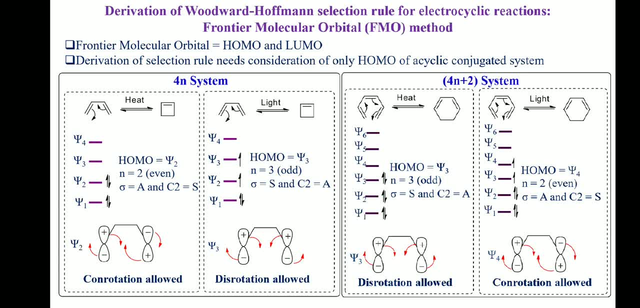 Under photochemical condition, one of the two electrons from psi 2 enters psi 3, making psi 3 as homo, Since n is equal to odd for psi 3, so it will have sigma plane and will not have C2 axis of symmetry. 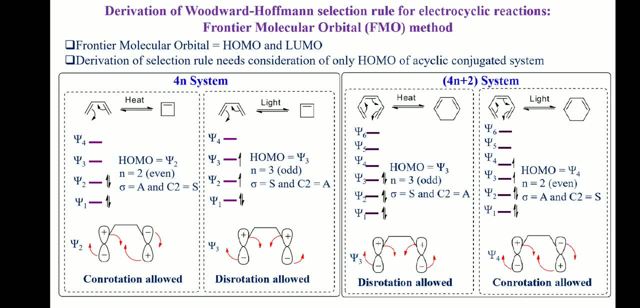 The structure of homo is such that the orbital lobes on the terminal carbons need to rotate in the opposite direction to form the cyclic product That is. the allowed rotation will be this rotation. In 4n plus 2 pi system, the case is reversed. 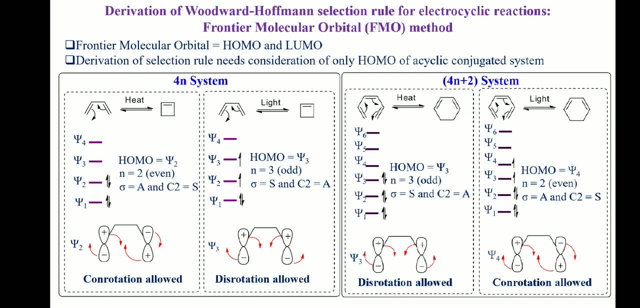 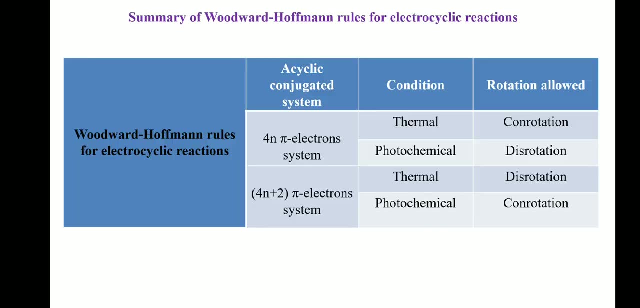 Under thermal condition, the homo has plane of symmetry, so the allowed rotation will be this rotation. Under photochemical condition, homo has C2 axis of symmetry, so the allowed rotation will be con rotation. Based on these discussions, we can conclude that the rotation of the orbital lobes is: 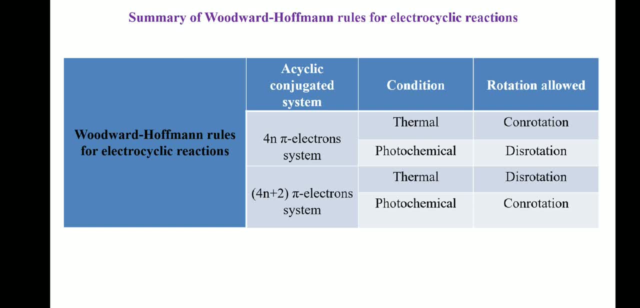 non-Engational. Based on these discussions, we can summarize Oudward-Halfman rule for Electro-Cyclic Reactions as shown in the table For a cyclic conjugated system with 4n pi electrons. under thermal condition the allowed rotation is related to con, but under photochemical condition the allowed 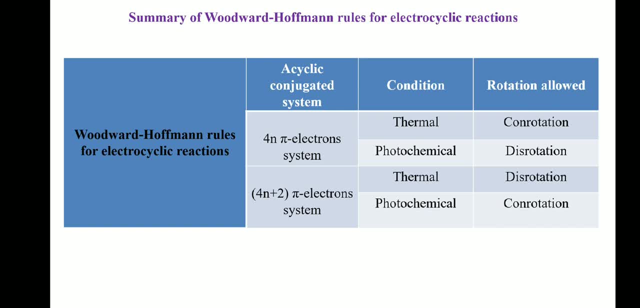 tooth rotation is related to dis Jess. For an afflictive Давis this rotation will beு sounds fucked up, I think- 4n plus 2 pi electrons. under thermal condition the allowed rotation is this, while under photochemical condition the allowed rotation is gone. 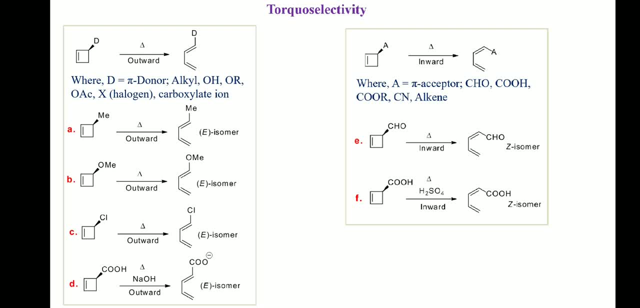 Now we are going to discuss torque selectivity in electrocyclic reaction. During electrocyclic ring opening process. pi donor substituents, like alkyl, OH, methoxy halogens, tend to move outward to minimize the repulsive interaction with the pi system. 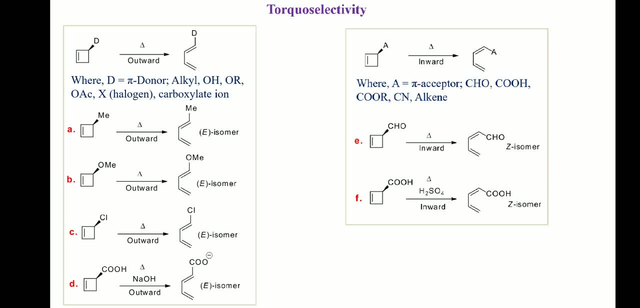 of polyene in the transition state, while pi acceptor substituents like aldehyde, carboglyc acid, ester, cyano, olefins, etc. tend to move inward of the polyene chains to stabilize the transition state by the interaction. 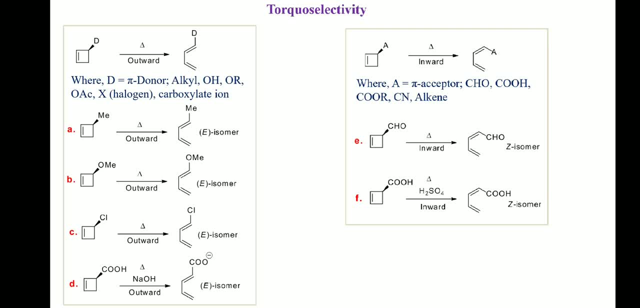 with the donor lobes of the p orbitals of breaking sigma-part. This preferential movement of substituents during ring opening is called torque selectivity, For example in reaction A, B and C because of the pi donor tendency of methyl methoxy. 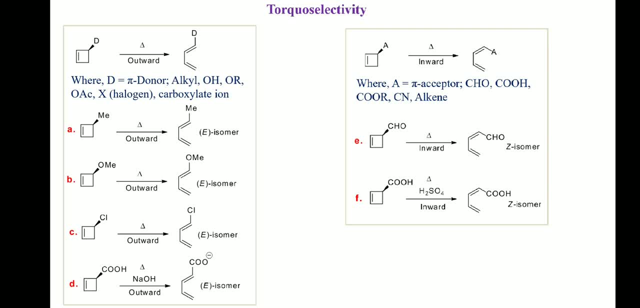 and chloro: 0, outward movement of groups resulted in the formation of E isomer over Z isomer In reaction D. outward movement of carboxylate group occurred to avoid repulsive interaction between the negative charge and the pi bond in the transition state. 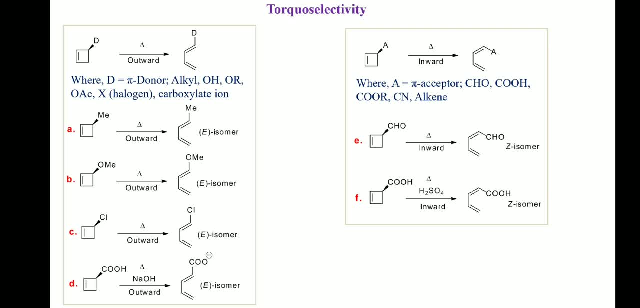 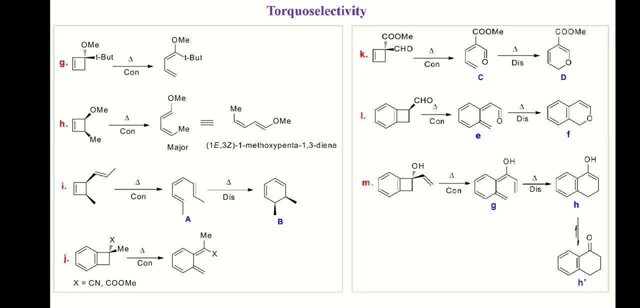 In reaction E and F. because of the pi acceptor tendency of aldehyde and carboxylic acid groups, inward movement of groups occurred that resulted in the formation of Z isomer over E isomer. Electronic factor dominates over the steric factor during the electrocyclic ring opening. 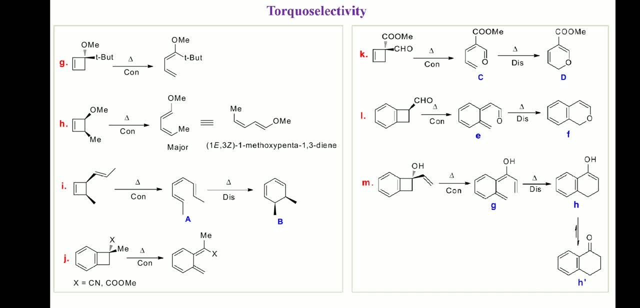 process. For example, in reaction G the strong electron-donating methoxy group moves outward, forcing bulky third butyl group to move inward. In reaction H the substituents at three and four positions are cis to each other. Open chain conjugate has 4n system, so under thermal conditions the allowed rotation will. 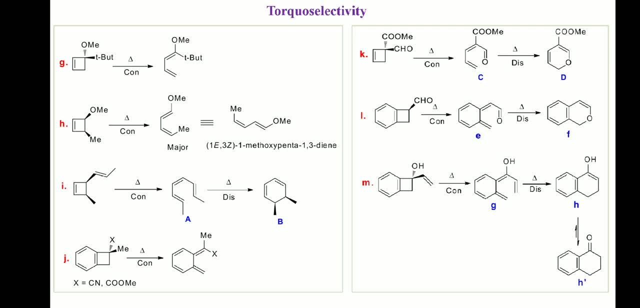 be conned and thus, after ring opening, both the groups will point in the same direction. This will be achieved when one group moves inward while other- outward- Methoxy group with strong donor tendency- moves outward, forcing methyl group to move outward. In reaction Z, the substituents at three and four positions are cis to each other. 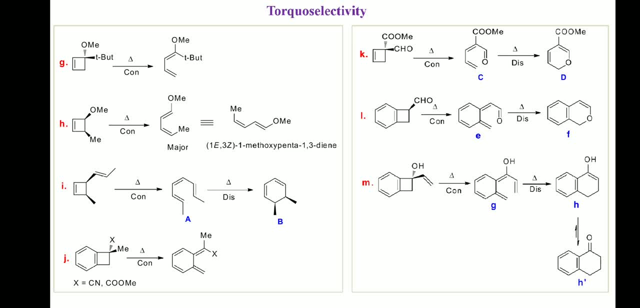 In reaction H, the substituents at three and four positions are cis to each other for inward rotation. in reaction I, inward movement of vinyl group during con rotatory ring opening process resulted the formation of intermediate a which, being for n plus 2 pi electron system undergoes this rotatory ring closing. 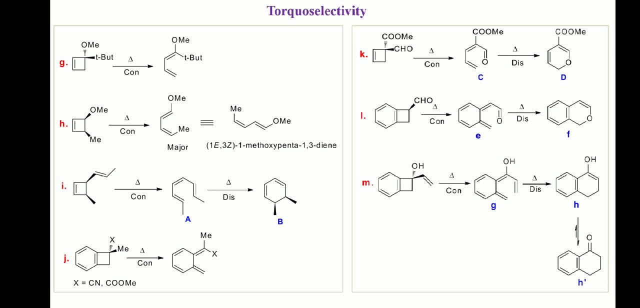 process to produce product B. in reaction j, during ring opening, electron donor methyl group moves outward, while acceptor nitrile or ester group move inward, according to the nature. when both the pi acceptors are present at C 3 position in word con, rotatory motion of the less bulky substituent takes place. 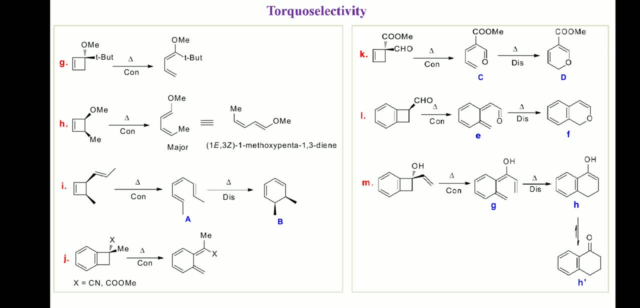 for example E In K aldehyde and ester. both are pi acceptors, but less bulky aldehyde groups move inward during conrotatory electrocyclic ring opening to form C which, being a 4n plus 2 pi electron system, undergoes disrotatory electrocyclic ring closing process to form product D. 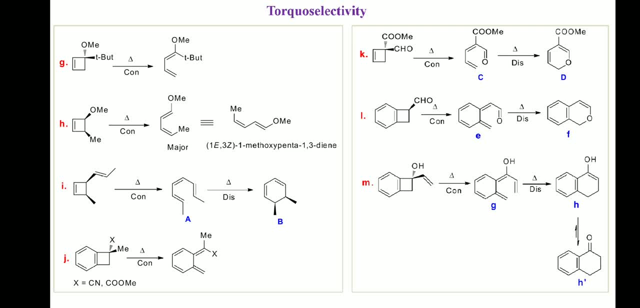 Similarly, formation of intermediate E and product F in reaction L can be explained In reaction M. according to the nature of the substituent, inward movement of the vinyl group and outward movement of hydroxy group leads to the formation of intermediate G which, being 4n plus 2 pi electron system undergoes disrotatory ring closing process. 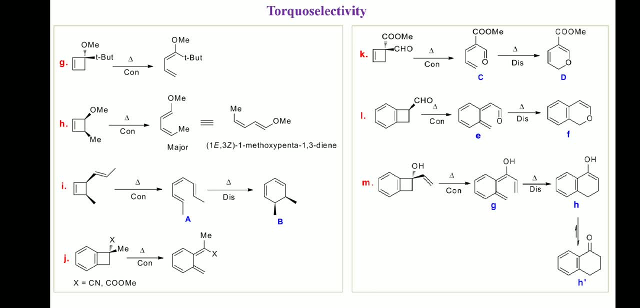 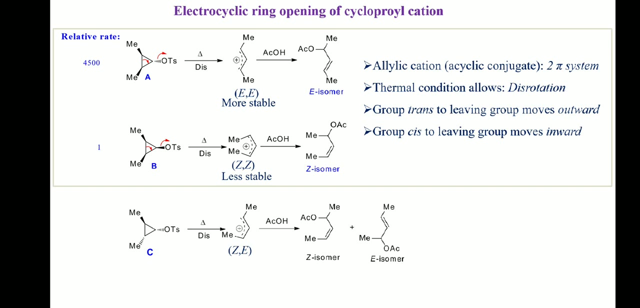 Electrocyclic ring closing process to produce product H. Product H after keto in ultratominism converts to form stable keto form H'. Electrocyclic ring opening of cyclopropyl cation. Rearrangement of cyclopropyl cation into allyl cation is an example of a smallest ring system capable of undergoing electrocyclic ring opening process. 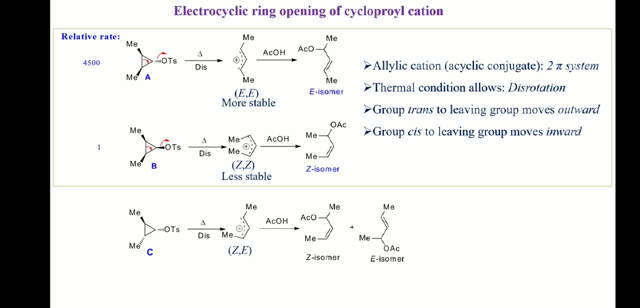 is, allyl cation has 2 pi electrons, or we can say 4 and plus 2 pi electrons. So according to Woodward-Hartmann rule, the process will be disrotatory under thermal condition. For more detailed discussion, let us take the example of. 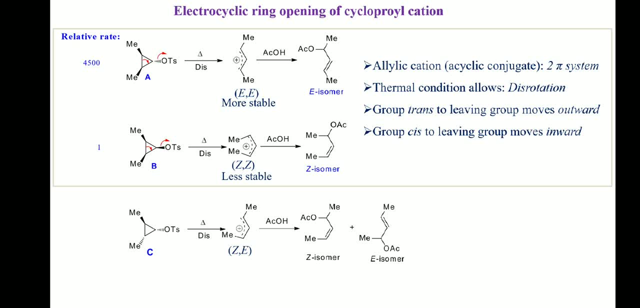 acetylysis of 1-tocyl-2,3-dimethyl cyclopropane. The orientation of leaving group affects the rate and stereochemical outcome of the reaction. Acetylysis of A having leaving group trans to the methyl groups is 4500 times.